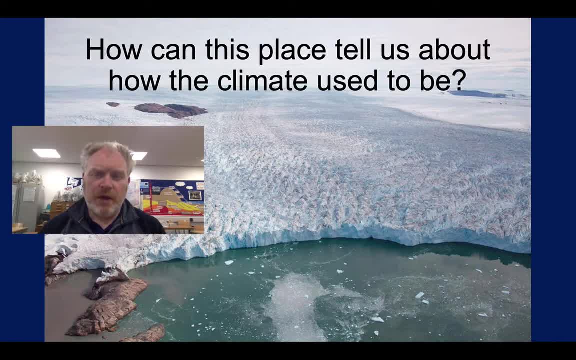 Hi, I thought I'd start with this photograph of an Antarctic ice sheet And with the slightly odd question: how can this place tell us how the climate used to be, And how can it tell us about the climate in other places? To answer this question, we need to use an idea we've. 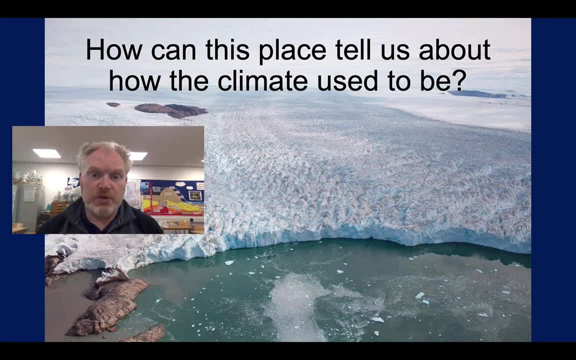 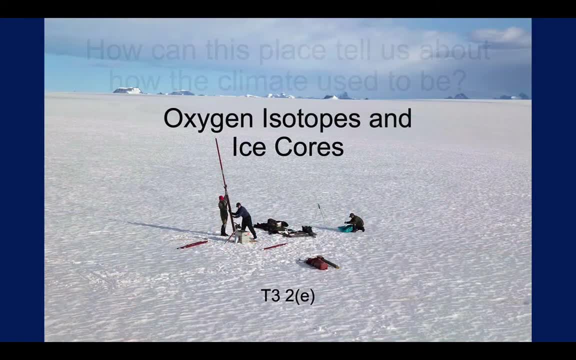 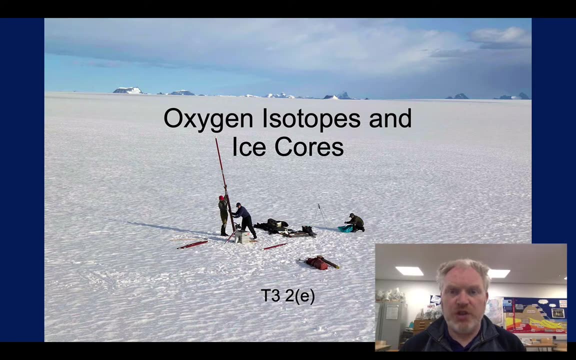 talked about before oxygen isotopes, but this time put it together with the record that we can find in ice cores. So these are records of ice that we drill from ancient ice sheets, either in Antarctica or in Greenland, but particularly in Antarctica, that give 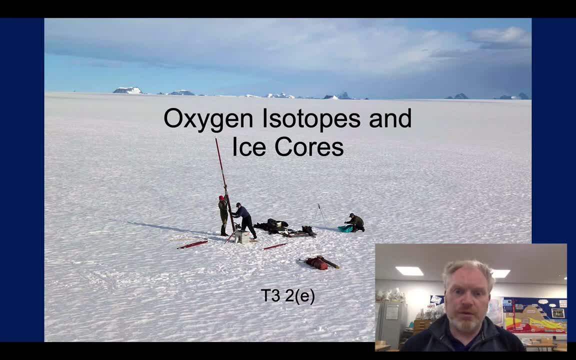 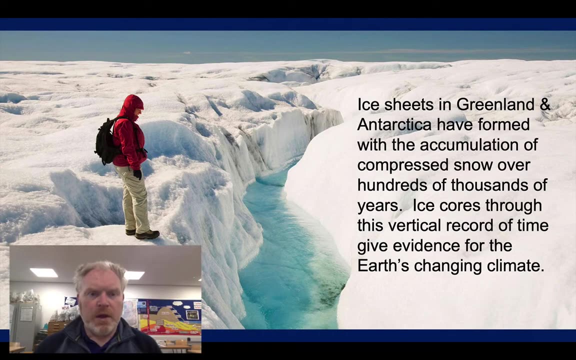 us a long geological record of ice Atmospheric composition and also the isotopic composition of the ice itself. The reason we do that in these places in Greenland and Antarctica is that we've had accumulation of snow which is compressed into ice over a significant period of time. 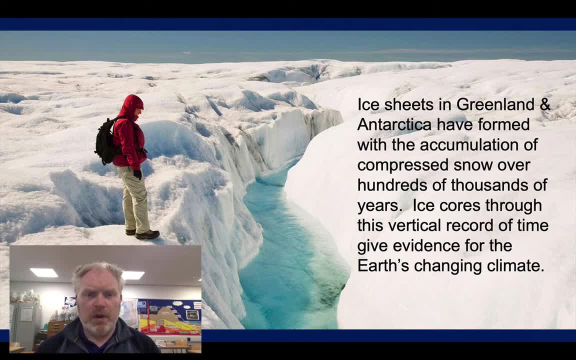 Hundreds of thousands of year long records, A record we simply don't get. from other ice sheets, For example, in the Alps, where the ice is moving far more, the ice is much, much younger, Maybe only thousands of years old. So the ice core records from these places give us this long, unbroken geological record. 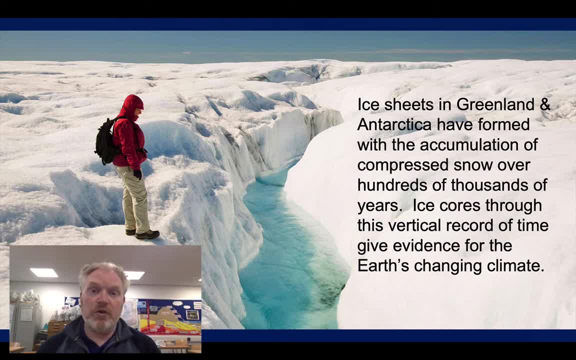 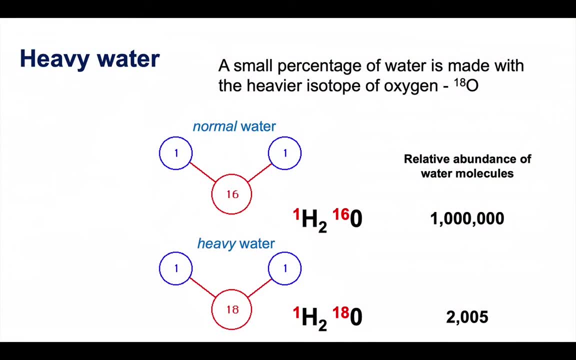 much in the way we'd get a long, unbroken record from cores of sediment from the deep ocean, Like the oxygen isotope data that we looked at for fossils from oceanic sediments. when we look at ice cores, it's based on a similar idea. You can see here we've got two isotopes. 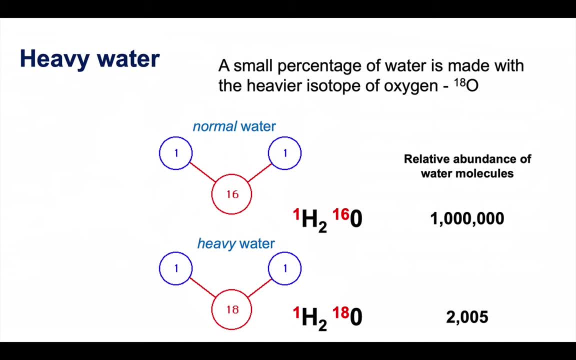 of oxygen. If you look, we've got normal water made of oxygen-16, that's very abundant- and then we've got a small proportion of heavy water, Water with this oxygen-18 isotope. Now, these two forms of water, we can't recognise the difference, but chemically they are slightly. 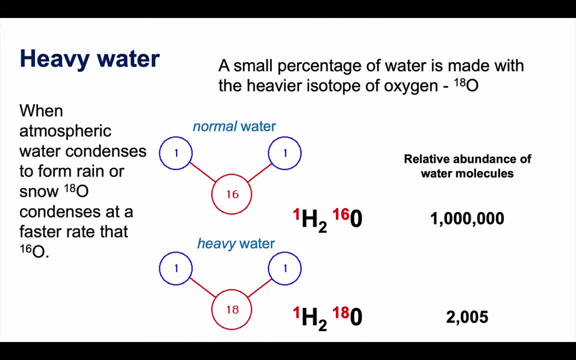 different, Behaves slightly differently And in particular it's the increase in the amount, increased likelihood of oxygen-18 condensing to form rain or snow, or it happens at a faster rate, should I say, than normal water. that means we get a response from the isotopic. 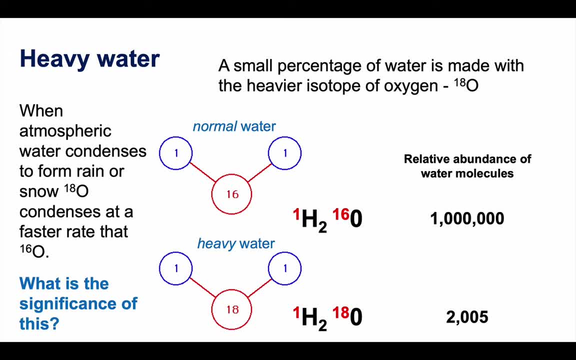 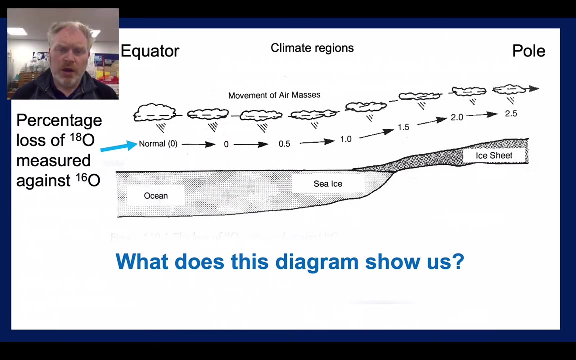 composition to changes in climate. What this means is we have a record of the climatic changes preserved within the water that actually makes up the ice, So let's think about the implications of this. You have this diagram as part of your handouts and it's a bit of. 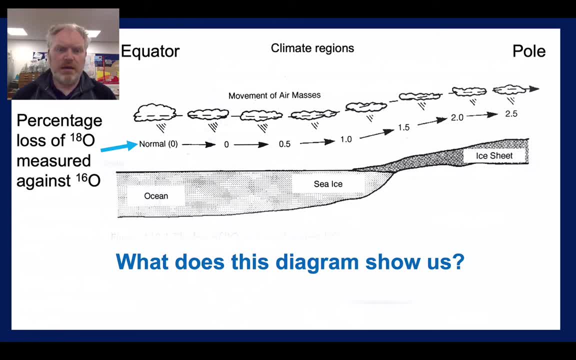 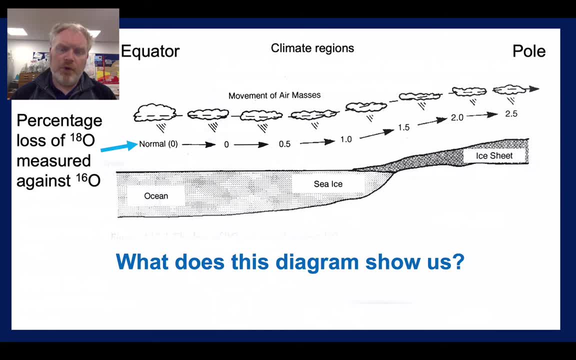 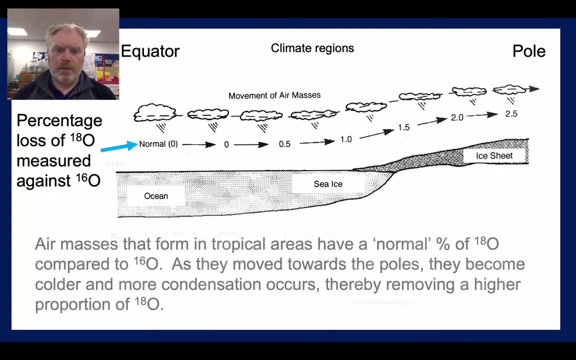 that falls as precipitation changes as we go from the equator to the pole, Progressively losing more oxygen-18 from the system as the temperature decreases. So if we look at the moisture in the air that forms around the equator, that has the normal percentage, the normal balance of oxygen-16. 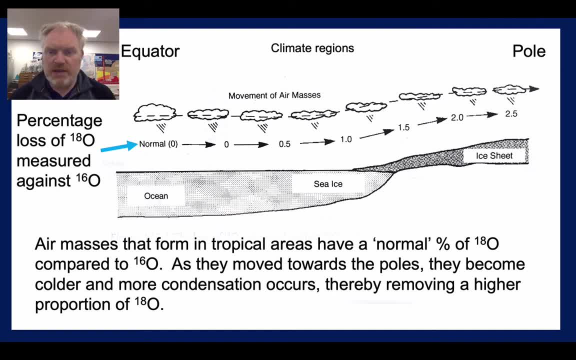 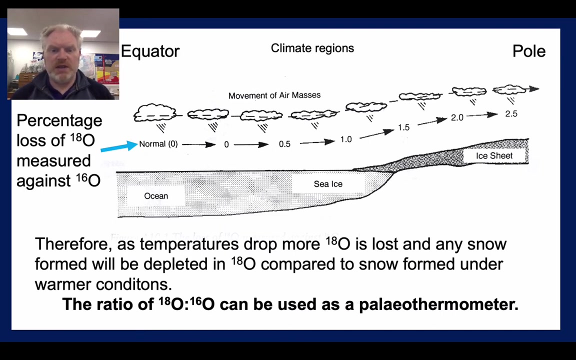 to oxygen-18.. As the air masses move towards the pole, they become more colder, so there's more condensation, more rainfall, and that will remove a greater proportion of oxygen-18 from that rain, from that snow, than we might expect. So as temperatures drop and we lose more of this oxygen-18, the snow that's. 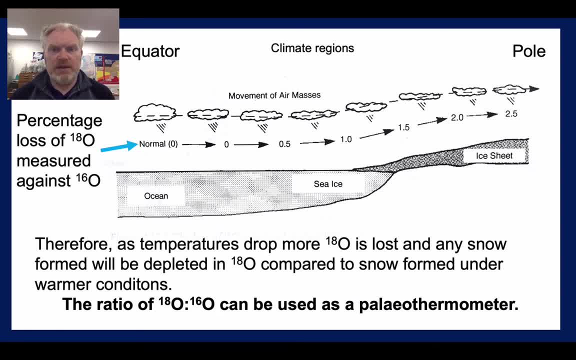 preserved in the ice sheets of the poles is depleted in oxygen-18, in the air, and these are driven out by the radiation that grows up. So we've now got an additional layer here that's enriched in oxygen-16, compared to snow or rainfall. 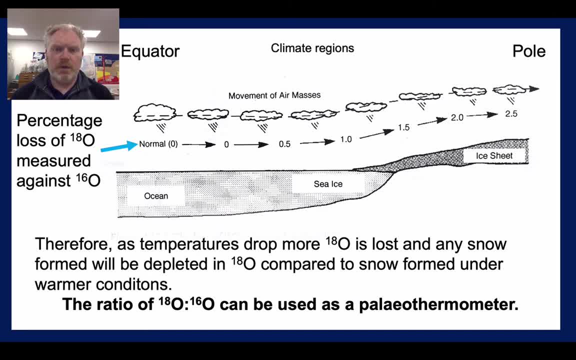 that's formed elsewhere, In particular. here we talk about snow, because that's what we get preserved. We don't get rainfall preserved. The upshot of all this is that this balance between oxygen-16 and oxygen-18 can be used. 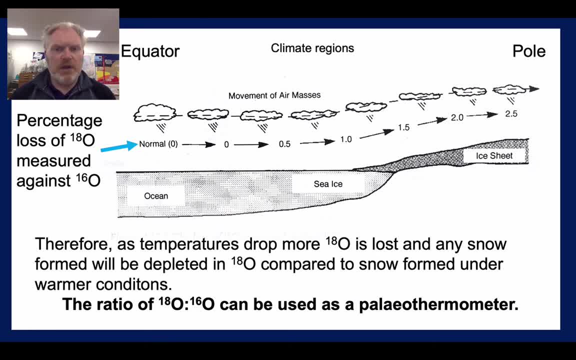 as a paleo-thermometer, Similar in a way to the way we use it in fossil shells, but Where we have colder conditions, we have more oxygen. 60. Because, remember, we're looking here at what's coming out of the ocean. 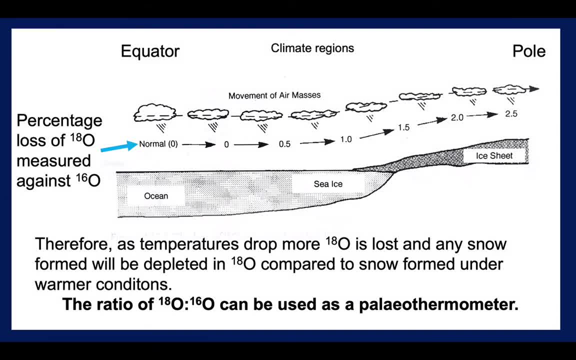 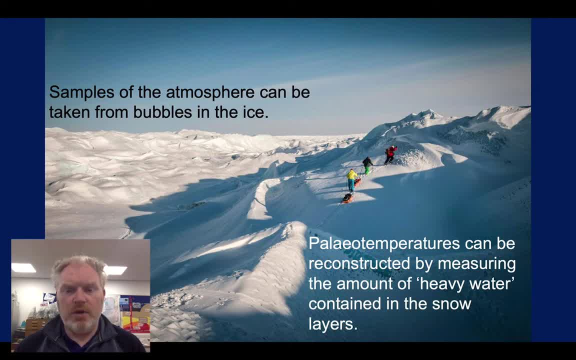 not what's left behind. So when we take an ice core, we can not only sample the snow and look at the isotopic composition of that snow, but we can also sample the atmosphere. Bubbles within the ice give us a sample of the atmosphere from the past. 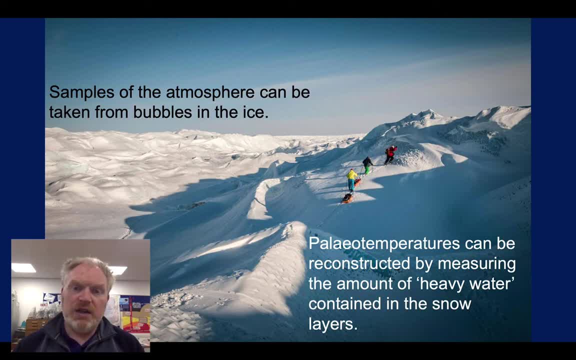 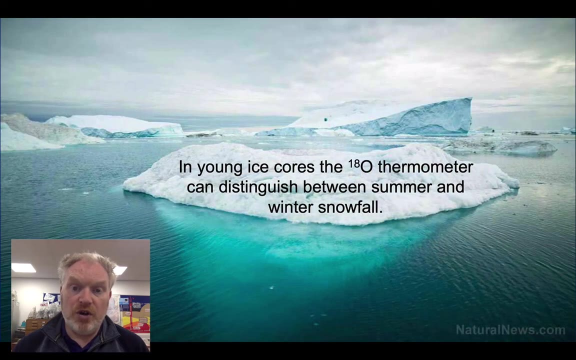 So we've got now a way of correlating these two climatic variables, temperature and also atmospheric composition. In really young ice cores, ones that are fairly recent, that haven't perhaps been compacted down, we can even detect seasonal differences, So we can see the differences between these. 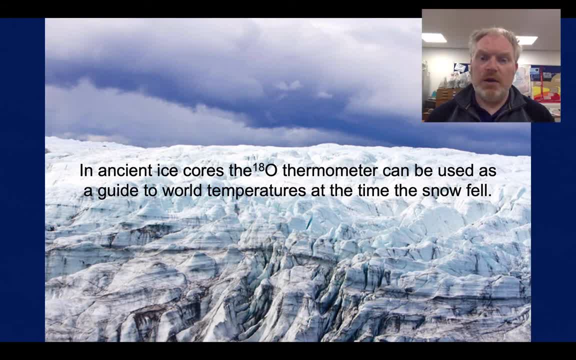 For the ancient ones, which is really what we're interested in. we can start to look at world temperatures. We get a global thermometer to track climatic changes over time and to correlate it with some of the other evidence that we get for these climatic changes.